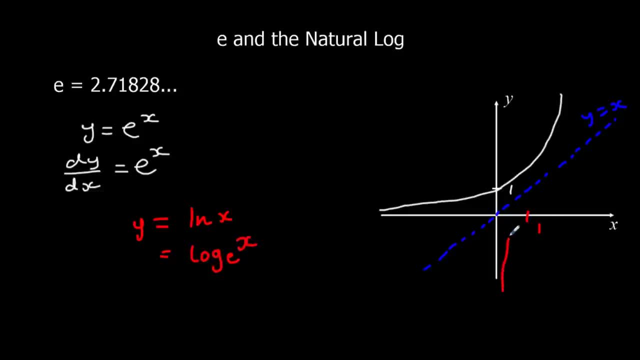 So this one comes up, never touching the y-axis, And it's a reflection in the line y equals x. So this is the graph of y equals ex, And this is the graph of y equals lnx. Now we're going to look at solving equations with e and ln. 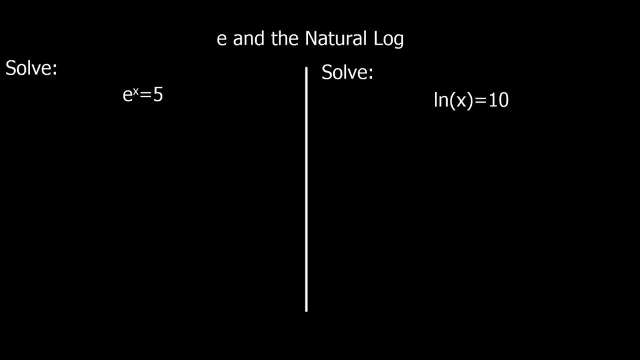 When we're solving equations, we use e and ln as the inverses of each other to solve equations. So here we've got a question: e to the power of x equals 5.. So to solve this, we apply ln to both sides. 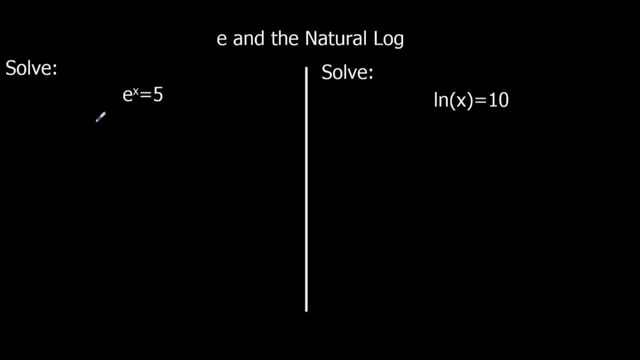 So we get rid of e by applying ln. So we get rid of e by applying ln to both sides. So ln e to the power of x equals ln 5. And then ln e just cancel out. So that leaves us with x equals ln 5.. 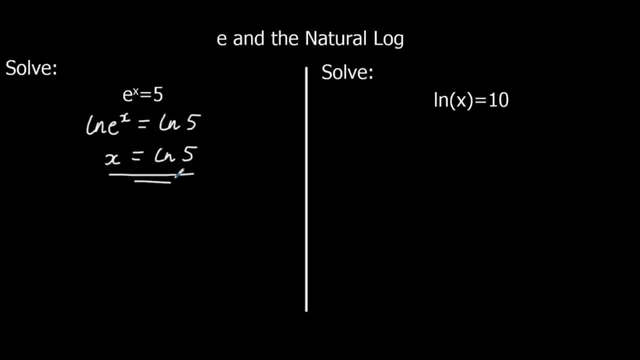 The other question. here we've got ln- x equals 10.. And we get rid of ln by applying e to both sides. So e, ln, x equals 10.. Then ln x equals e to the power of 10.. eln cancels out, which leaves us with x equals e to the power of 10.. 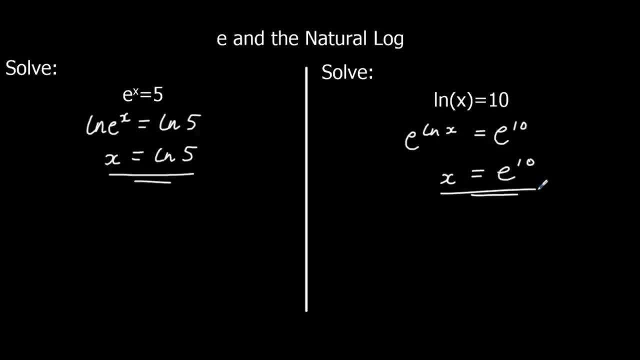 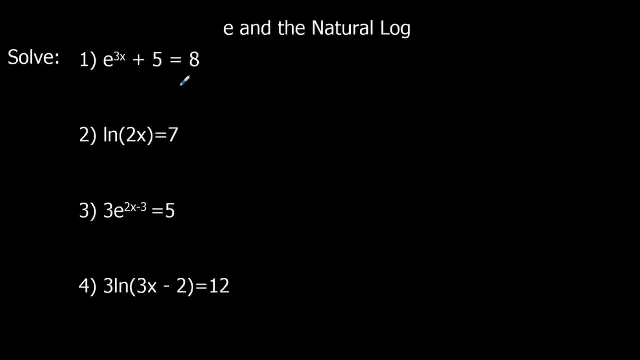 So we use the factor e and ln at the inverse of each other to solve equations. The first question here: we've got e to the power of 3x plus 5 equals 8.. So the first thing we're going to do is we're going to get rid of the plus five. 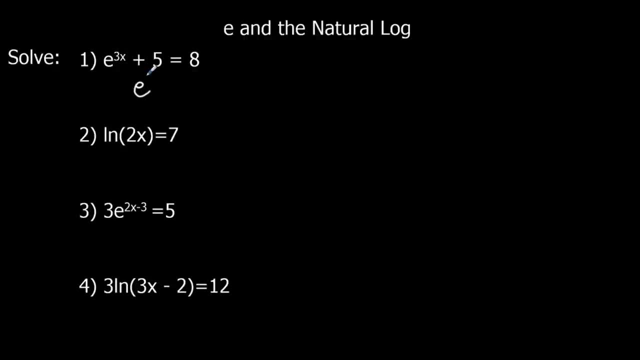 by taking the e to the power of 6. 5 from both sides. so that will give us e to the power of 3x equals 3. now we're going to deal with the e. so to get rid of an e, we're going to apply ln to both. 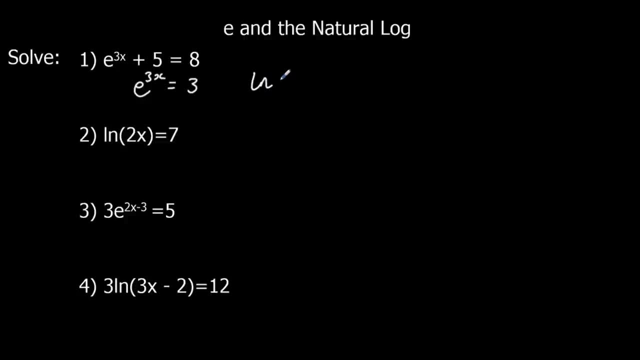 sides. so ln e 3x equals ln 3. on the left side now we've got ln e and that is going to cancel out ln e cancels out. so that's 3x equals ln 3. and to get x by itself, we're going to divide both sides by 3, so x equals ln 3 over 3. okay, the. 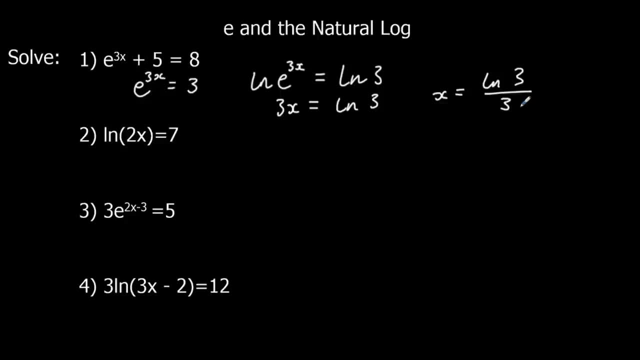 second question: so we've got ln 2x equals 7. so this time we're going to get rid of ln by applying e to both sides, so that's e. ln 2x equals e 7. e ln is going to cancel out, so that would be 2x. 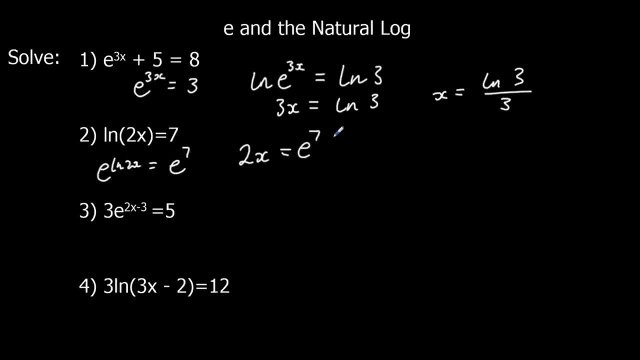 equals e to the power of 7, and then I'm going to divide both sides by 2, which will give me e to the power 7 over 2. okay, question 3: we've got 3 e to the power of 2x minus 3 equals 5.. So we're going to get rid of the 3, first by dividing both sides by. 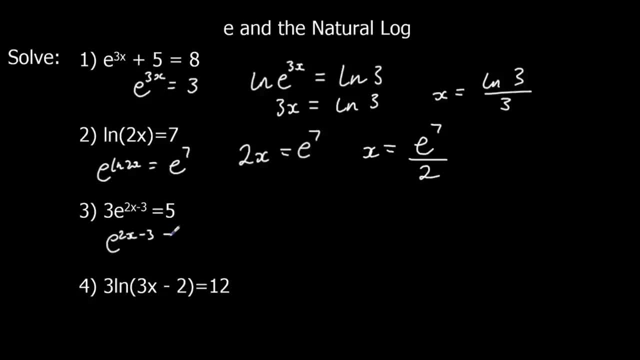 3. So e 2x minus 3 equals 5 thirds. And then we're going to apply ln to both sides, So ln e 2x minus 3 equals ln 5 thirds. ln e cancels out, So we've got 2x minus 3 equals ln 5 thirds. We want a plus. 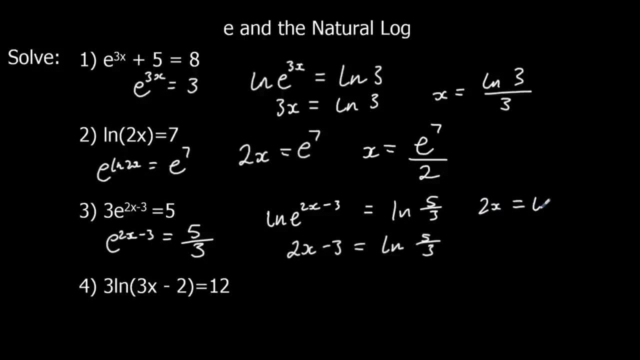 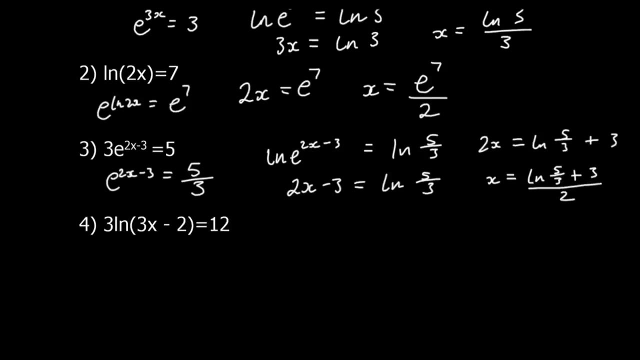 3 to both sides. So 2x equals ln 5 over 3 plus 3, and then divide by 2. ln 5 thirds plus 3 all over 2. And finally we've got 3. ln 3x minus 2 equals 12.. So we're going to divide by 3 first. 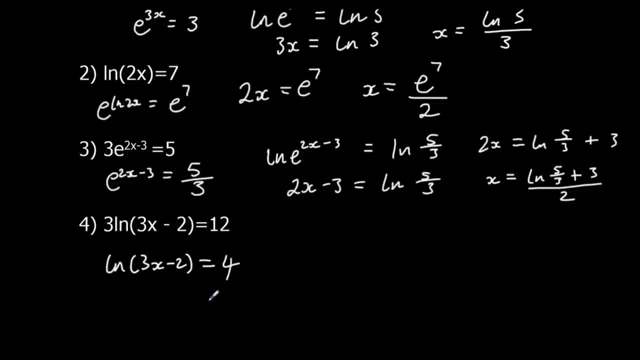 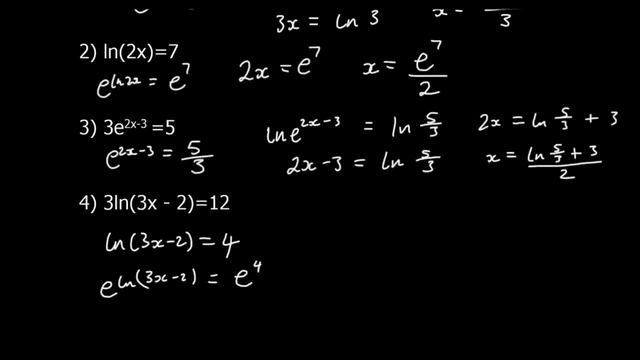 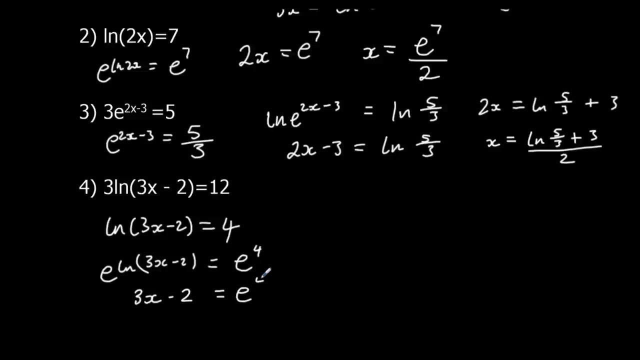 ln 3x minus 2 equals 4.. And then we're going to apply e to both sides, So e ln 3x minus 2 equals e to the power of 4.. Now e ln cancels. So we've got 3x minus 2 equals e to the power of 4, plus 2 to both sides, e to the. 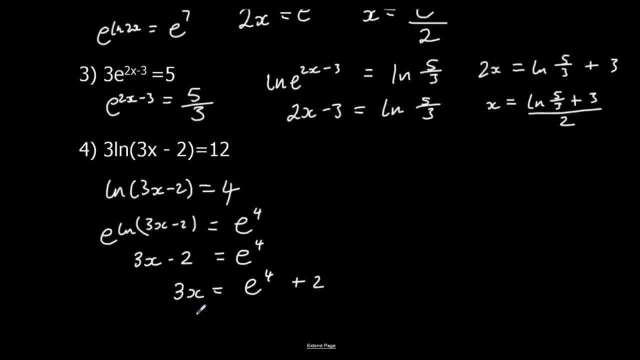 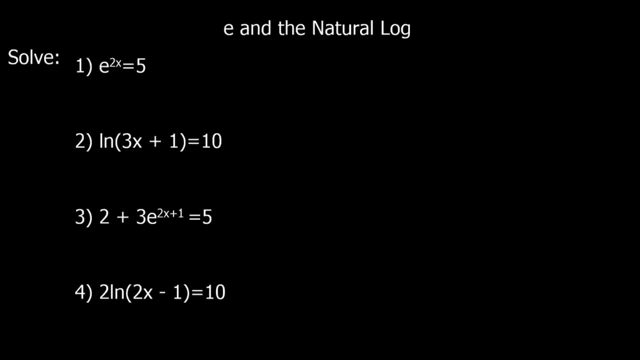 power of 4 plus 2 is equal to 3x and divide by 3.. e to the power of 4 plus 2 over 3.. Okay, here's some more questions. Pause the video, give them a go and I'll go through the answers. 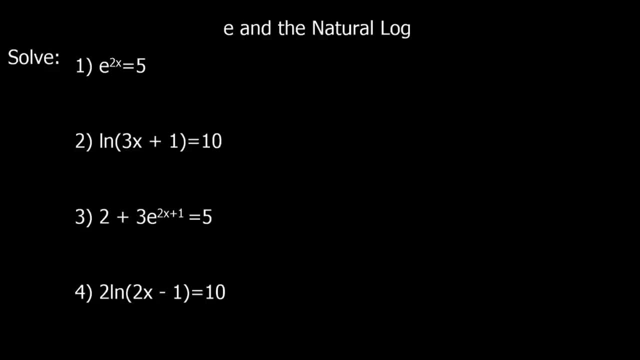 after: Okay, so the first one: we've got e to the power of 2x equals 5.. So we're going to get rid of e by applying ln to both sides, So ln e 2x equals ln 5.. ln e cancels, So that's 2x equals ln 5 and 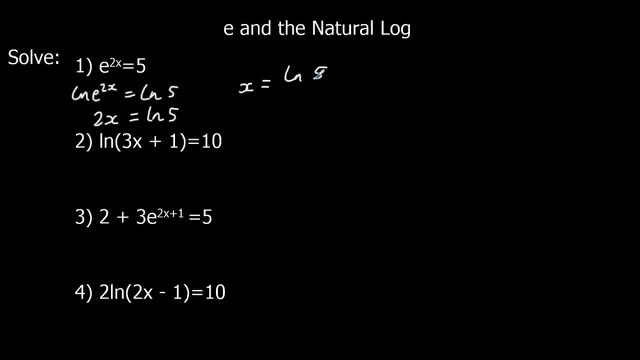 then divide both sides by 2.. So x equals ln 5 over 2.. Secondly, we've got ln 3x plus 1 equals 10.. So we're going to get rid of ln by applying e to both sides. So e ln 3x plus 1 equals e to the power of 10. e ln cancels. So we've got 3x plus 1 equals. 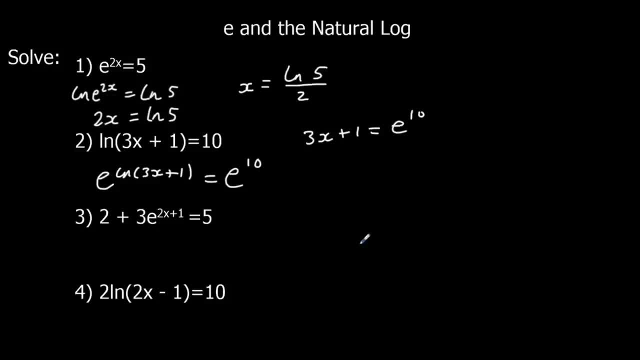 e to the power of 10.. Then we want to take 1 from both sides, So 3x equals e to the power of 10 minus 1.. And divide by 3 finally, So e to the power of 10 minus 1 over 3.. 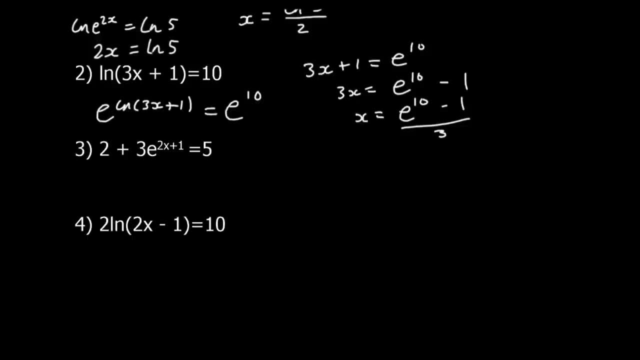 Question 3.. 2 plus 3e to the power of 2x plus 1 equals 5.. So the first step we're going to take away 2 from both sides, So 3e to the power of 2x plus 1. 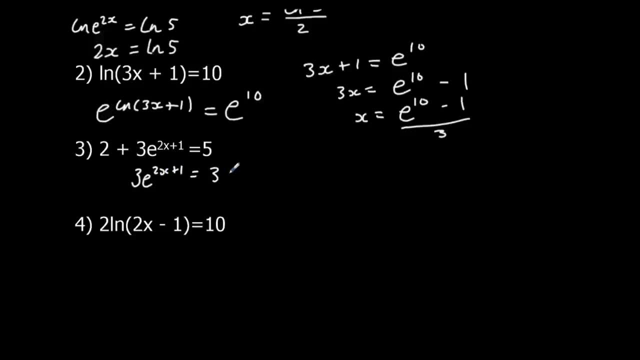 equals 5.. equals 3.. Then we're going to divide both sides by 3, which is going to give us just e. 2x plus 1 equals 1.. Now we're going to get rid of e by applying ln to both sides, So we've got ln. 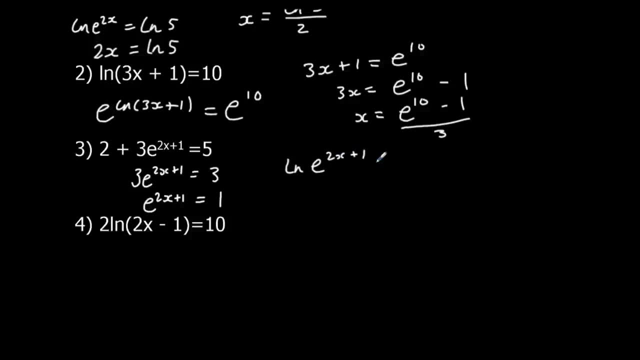 e 2x plus 1 equals ln 1.. ln 1 is actually 0, so we can change it to 0.. But ln e cancels, which is 2x plus 1 equals ln 1.. But ln 1 is 0, because, if you remember the graph,